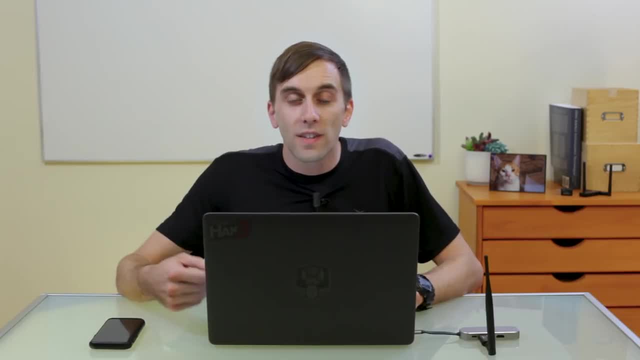 both to repeat themselves many times Now. using this technique enables you to, in a very short period of time, build up the information you need to crack the password and get into the network without any hassle at all. You can also use this technique to crack the password and get into the. 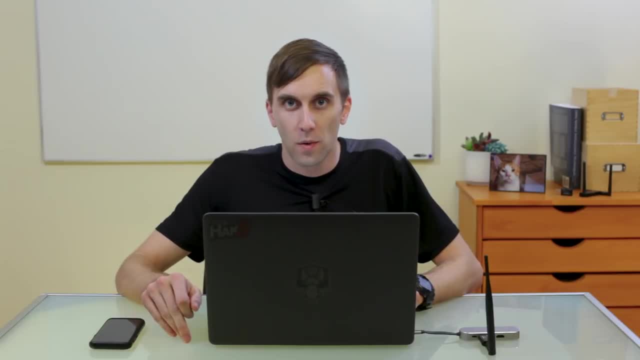 network without any hassle at all. So to do this we'll use two different tools. One is called AeroDumpNG, and we'll use this to take the data from the panda wireless network adapter, filter it so we only see WEP networks nearby, and use this as a filter for our next program, which is 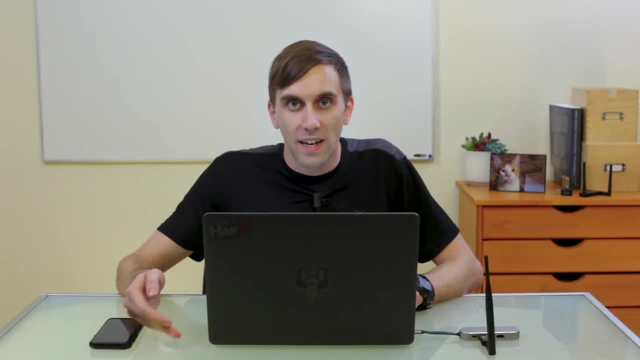 called B-SideNG. Now, B-SideNG we'll use to attack the network, because it's generally a network attacking tool that's very effective, but we'll need to give it some filter data, Otherwise it will go after every single network in the area and it's going to be a lot of work. 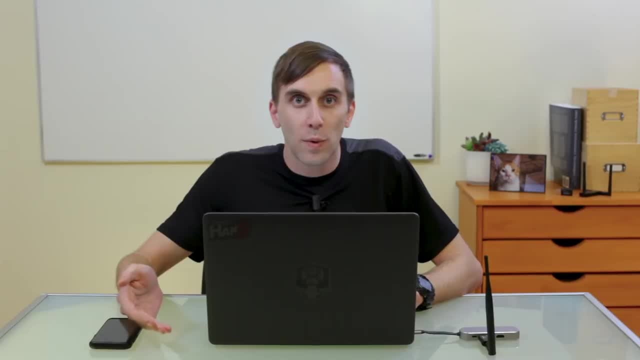 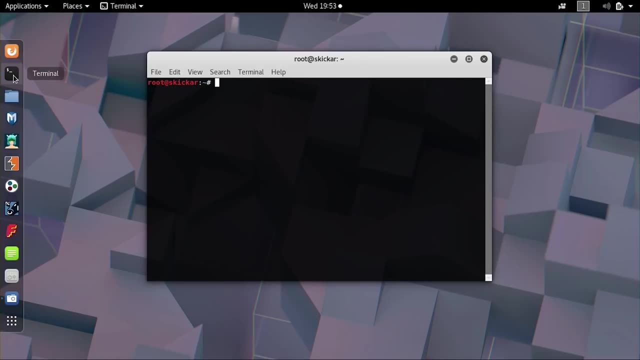 And that is not what we want. So this all seems pretty simple, and it is, So let's get started. Once you boot your Kali Linux machine, open a terminal window and plug in your network adapter. The first step will be to find the name of the network adapter, which you can do by typing: 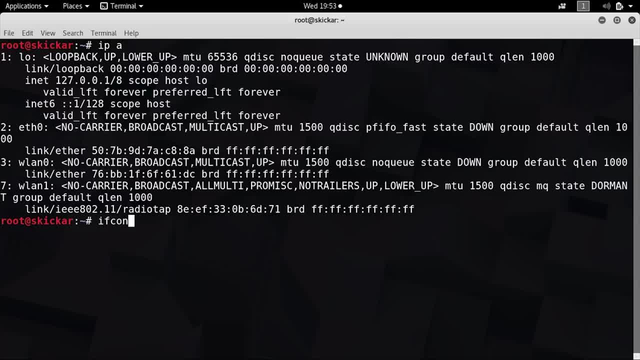 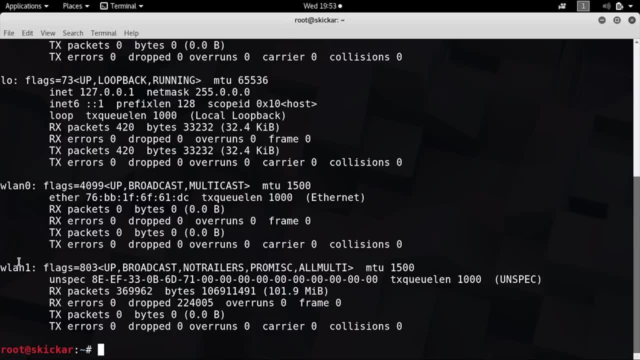 ipa or ifconfig. Here the name of our network adapter is wlan1.. We'll be using a program called AeroDumpNG to find any nearby WEP networks. So type AeroDumpNG and then tac, tac, encrypt WEP and press enter. 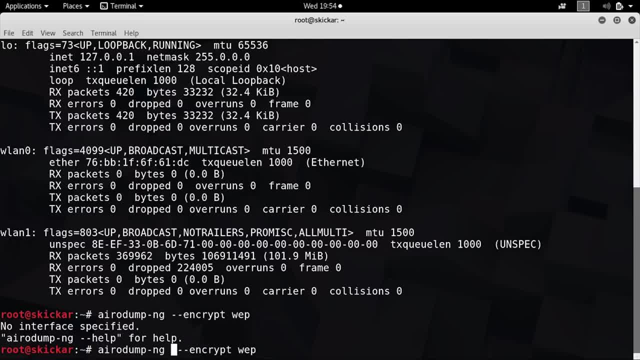 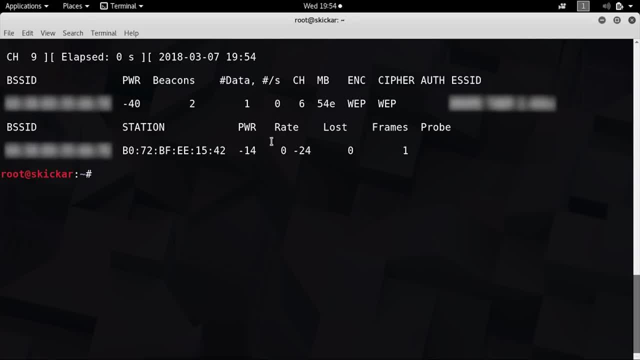 Oops, sorry, We'll also need to put in the name of our network adapter, So type in wlan1.. There we go Now, as you can see, it instantly found a network using a WEP connection nearby or WEP encryption nearby, So we'll go ahead and note the channel that it's on, which is channel 6,. 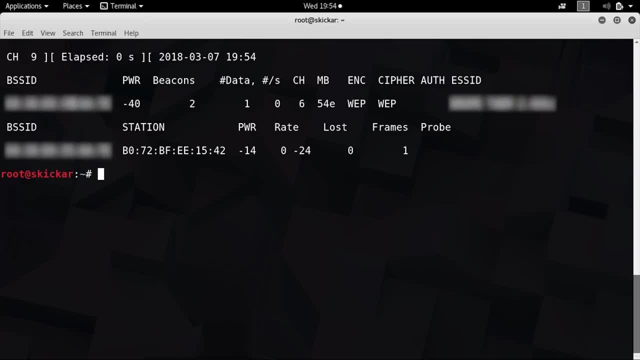 and then the BSSID, which is also the MAC address. So we'll copy this MAC address because we'll need it for the next step, in which we will tell BSideNG, a tool for attacking wireless networks, that we want to attack that network and only that network. 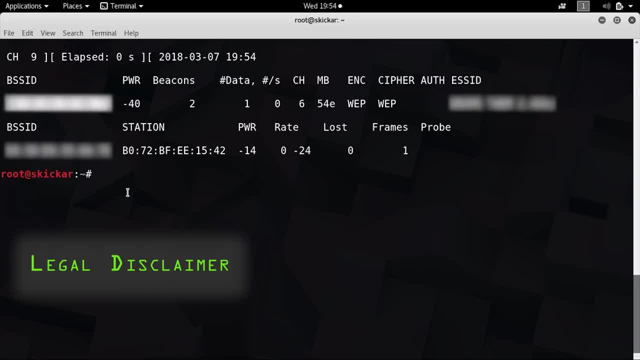 Now it's important for us to mention here that attacking a network that you don't have permission to can be a crime, depending on where you live. So you need to do this against a network you have written permission to audit, or your own network, in the event that you're just kind of. 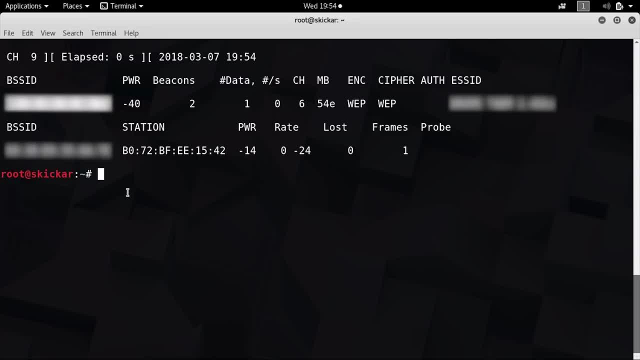 testing this out Now. WEP networks make a great honeypot, so make sure you're not cracking into anything you don't have permission to. Now to start BSideNG type BSideNG the name of the network adapter, wlan1, and then tack C for channel 6,. 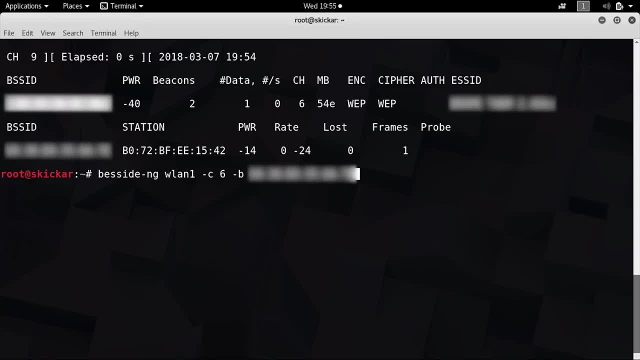 and tack B and paste the BSSID. So now, when you press enter, we should start injecting packets only for this one particular network, because if we didn't put BSideNG, BSideNG would just attack every single network nearby, in no particular order. 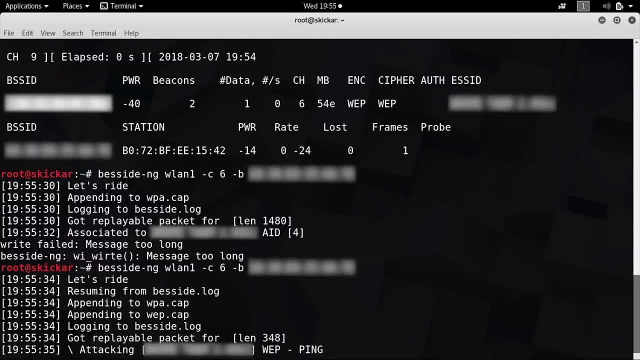 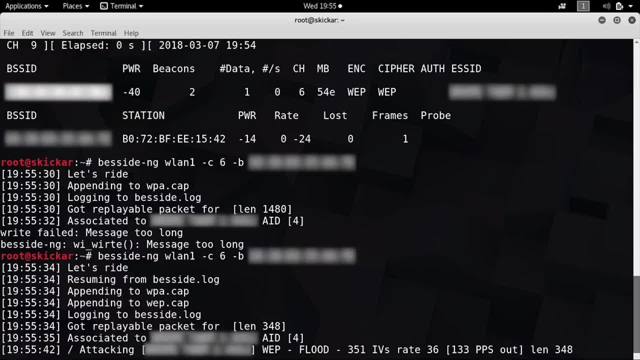 So after executing this, we can see that, after an initial hiccup, BSideNG is running and it's selected the correct network that we want to attack. So IVs are the type of packets that we can use to crack this password. 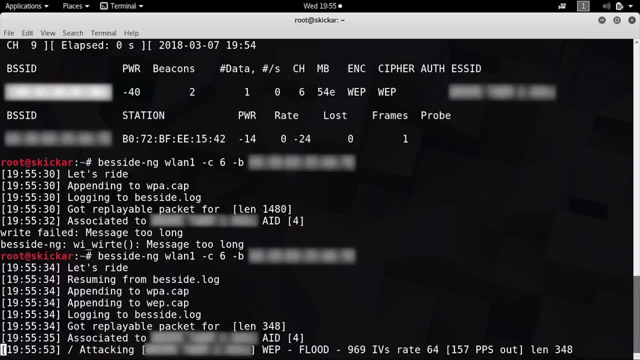 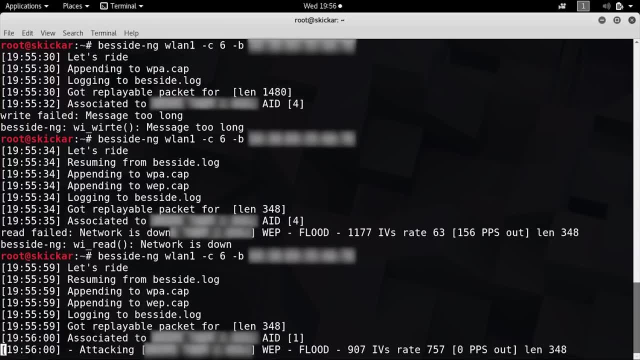 and BSideNG will continue to try to stimulate as many as possible, first with just injection but then with a flood. So if your network card goes down for some reason or if there's any other issue, you can generally just run the command again, because it's saving all these things to a cap. 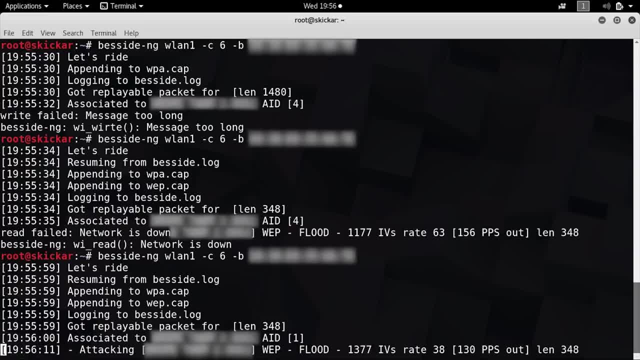 file which will save all the IVs that you are able to pull down from BSideNG. and if you're really having trouble with your network card, you can just run aircrackng to get both the hex version of the password which BSideNG will give you at the end of this process. 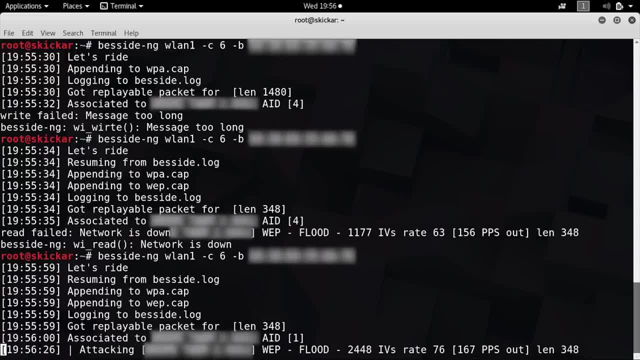 or it can also give you the ASCII version of the password, which is much, much easier for people to remember. So hopefully we'll be able to get a. oh, there we go. we'll be able to get a packet that allows us to flood and really create a ton of different IVs in our cap file, and it's important to note. 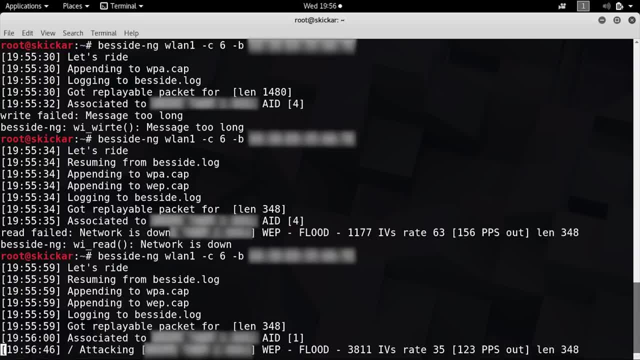 that this is going pretty fast. If you were a person who had this Adobe EP network, you probably should be worried that we would be able to get in here in less than five minutes, maybe even less than two minutes, because once somebody's on your network, 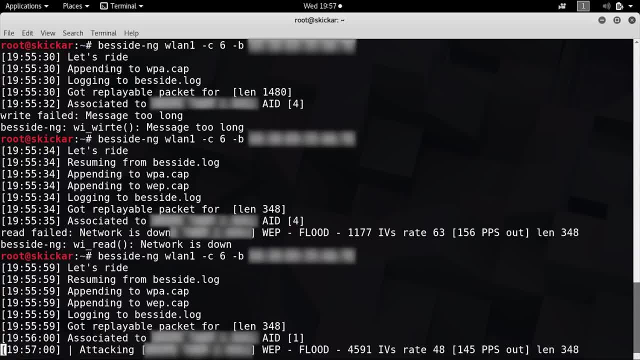 they can do things like a man-in-the-middle attack, which basically controls your internet experience, can route you to fake login pages, run key loggers and otherwise steal passwords and worm their way into your life even worse. So now you can see we're doing floodcracking.